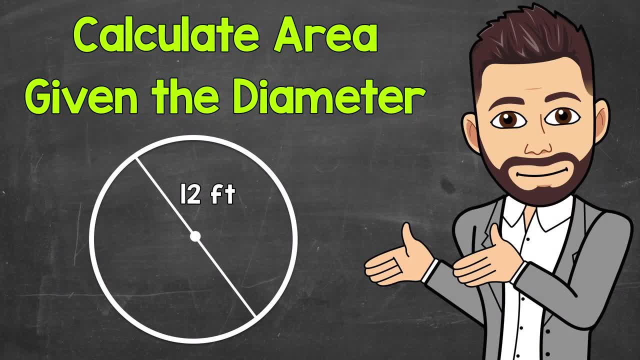 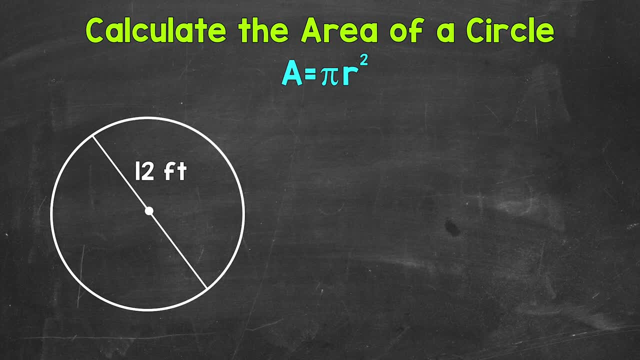 Welcome to Math with Mr J. In this video I'm going to cover how to find the area of a circle, given the diameter. Now remember: area is the amount of space a 2D figure takes up and we can measure in square units. 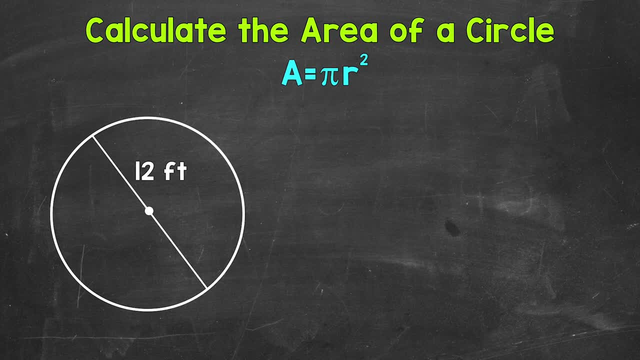 So how many square units does a given figure take up? Or you can think of it as how many square units to cover the given figure. Now the formula we use for the area of a circle is: area equals pi r squared, So pi times the radius squared. 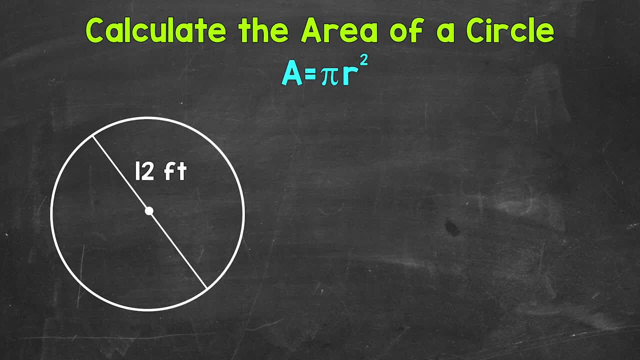 So we do need to be familiar with both diameter and radius when we work with circles. Diameter is the distance all the way across a circle, So it's a line segment that connects two points on the circle and it has to go through the center. 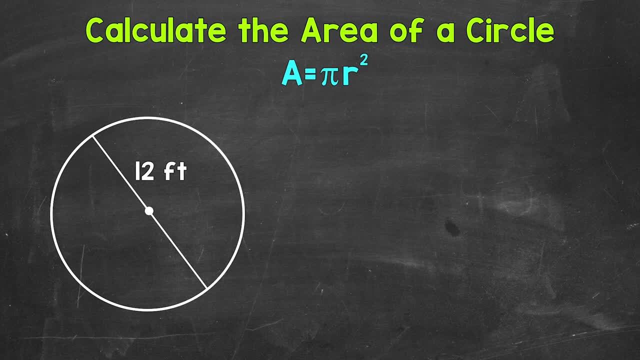 And then the radius is half, Half the diameter, So it goes from the center to any point on the circle. And then, lastly, before we get into our example, is pi, Which is the ratio of a circle's circumference to its diameter. 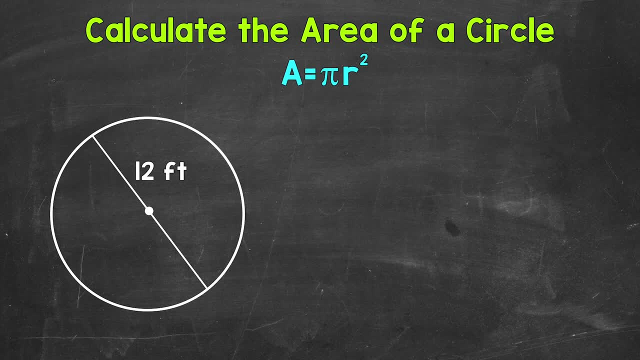 Pi is a constant, So it's the same for all circles. Now pi is irrational. It goes on forever. So we are going to use an approximate or rounded version of pi 3.14.. With that being said, let's jump into our example, where we have a circle with a given diameter of 12 feet. 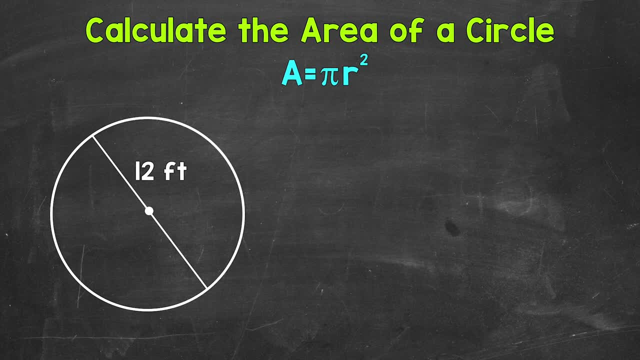 Now the first thing that I'm going to do is write out the formula for the area of a circle, So area equals pi r squared. Next we can plug in our radius, So area equals pi times. Now we are going to use a formula for the area of a circle. 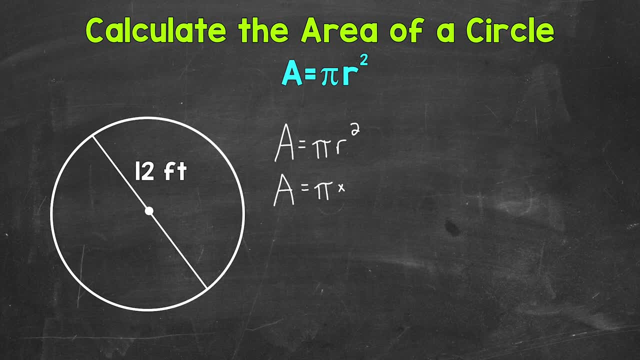 We are given the diameter, so we need to divide that diameter by 2 to get the radius, Because, remember, the radius is half of the diameter. 12 divided by 2 gives us a radius of 6 feet. Let's plug that in. 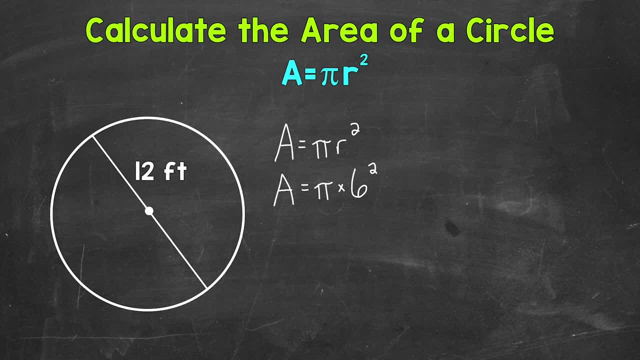 And that's going to give us 6 squared. Now, 6 squared, that means 6 times 6.. Not 6 times 2.. When we square a number, we multiply that number by itself. So let's do 6 squared, which gives us 6 times 6, which equals 36.. 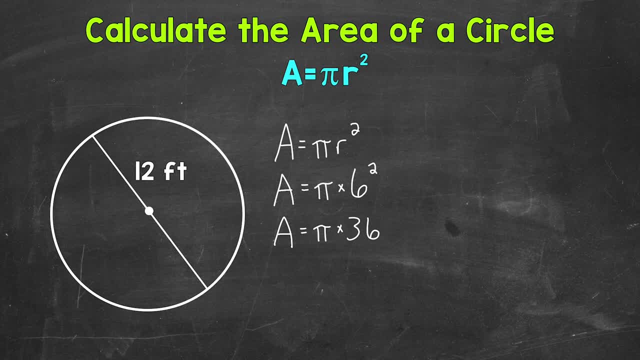 So we end up with pi times 36.. Now one way to write the area of a circle is to write it in terms of pi Meaning. we can write our number in front of the pi symbol and then put our unit of measure. So we can put 36 pi. 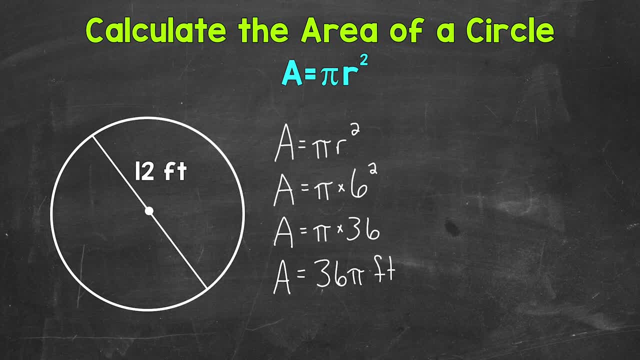 And this is square feet- Square feet for our unit of measure. So that's one way we can write out our area of that circle. Another option: we can use an approximate rounded version of pi. Like I mentioned earlier, we're going to use 3.14.. 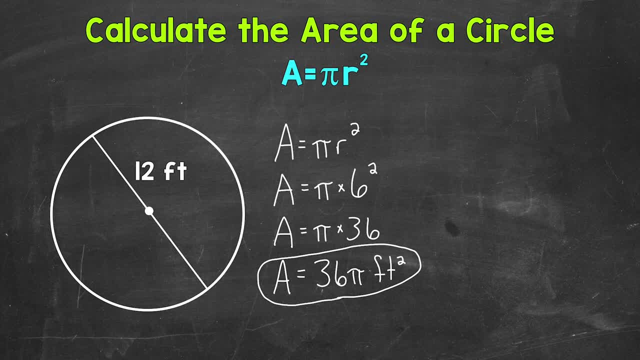 So we can use this to get an approximate area of the circle in decimal form. So again, we're going to use pi. Pi is approximately 3.14.. So that squiggly equal sign. that's the approximate symbol, Unlike an equal sign which means an exact value. 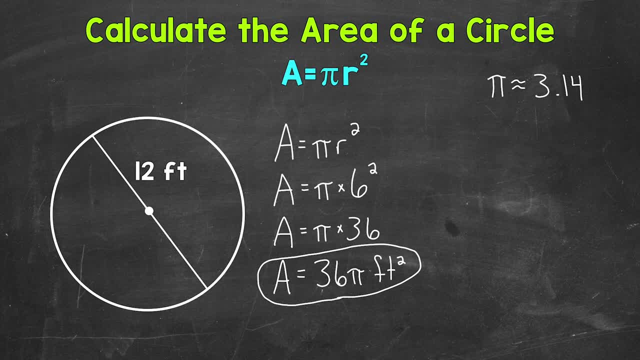 So something to keep in mind when you see that sign. Let's write out our formula, which is: area equals pi, r squared, And then we can plug in: So area is approximately. I'm going to use the approximate symbol there Because, again, we're using an approximate version of pi. 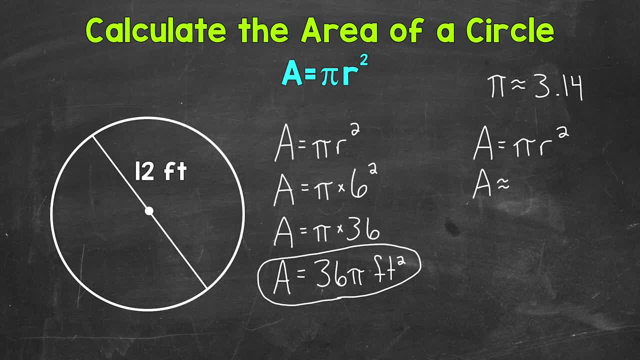 So we are going to get an approximate area. Let's plug in 3.14.. And then multiply by our radius, which is 6 squared, And now we can calculate here. Let's do 6 squared, So 3.14 times 6 squared, which equals 36.. 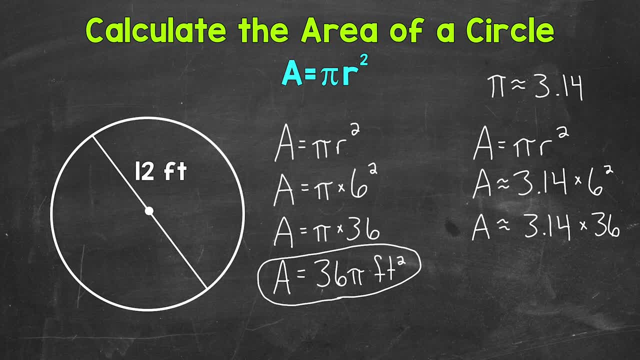 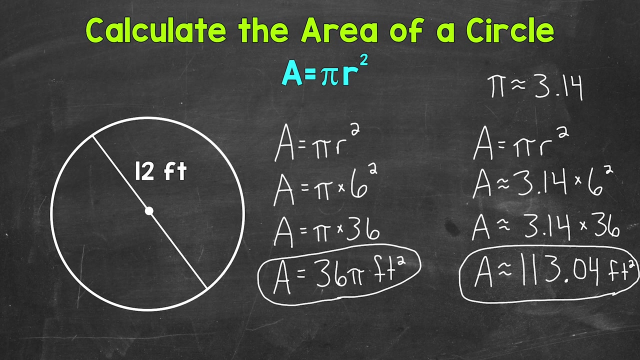 And now let's multiply. So 3.14 times 36 gives us an approximate area of 113 and four hundredths, And this is square feet. So that is an approximate area of that circle. So there you have it. There's how you calculate the area of a circle.